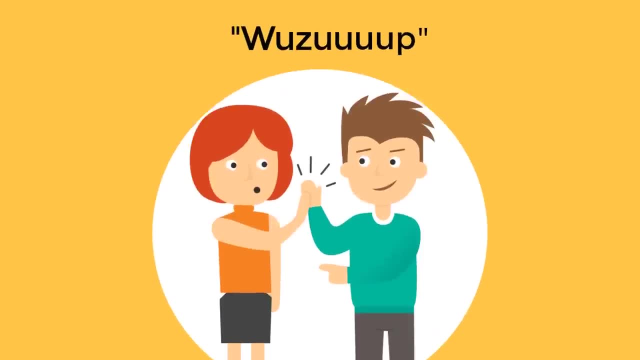 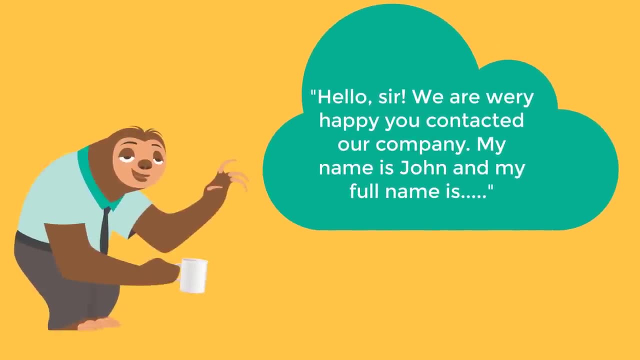 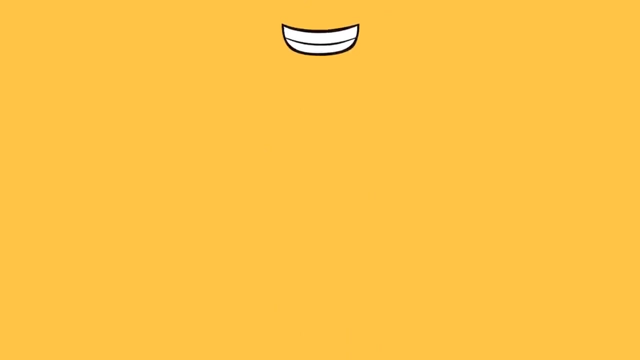 Either their greeting is too short and informal or too long and formal, both of which betray the lack of respect and concern for the customer. Greeting should be professional while remaining friendly and personal at the same time. A good example would be: Hello John. thank you for calling. Provide Support. how may I help you? 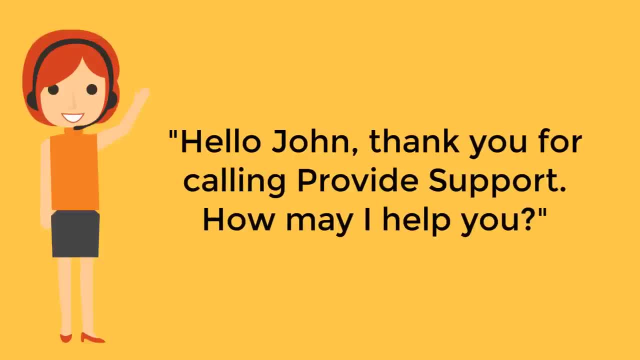 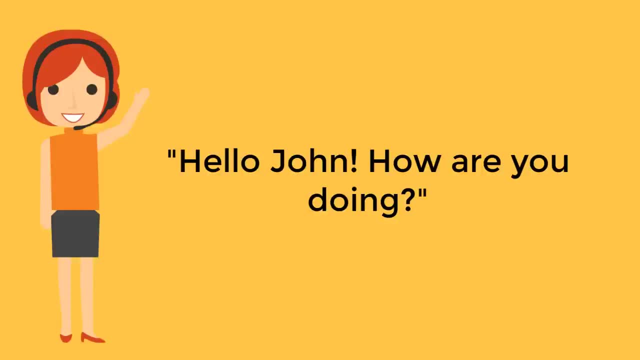 Or you can start with a shorter but more personal greeting: Hello John, how are you doing? Hello John, how are you doing? We like this one, as it works really well. Many customers are actually surprised by this question in a good way. 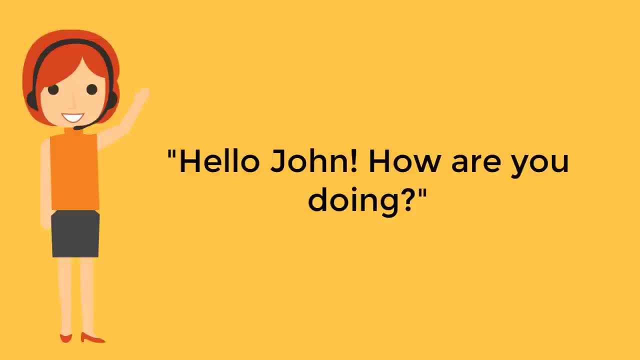 Probably because support elsewhere rarely asks them this question. It instantly sets the rep on friendly terms with the customer and the conversation becomes less formal and template-based, while keeping a business tone. After the customer confirms his well-being, you can move on with Perfect. I'm really glad to hear that. How may I help you today? 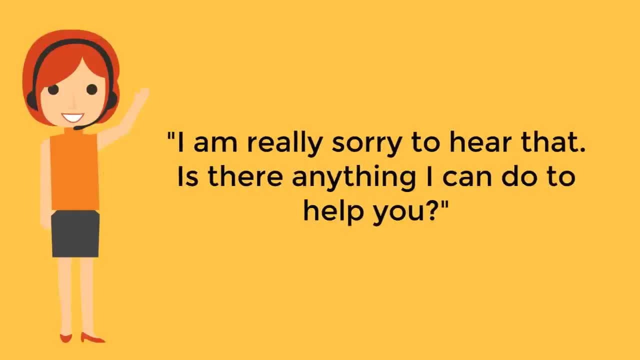 Or you can express your sentiment. You can express your sympathy if the customer is not doing well. I'm really sorry to hear that. Is there anything I can do to help you? If the customer starts the chat with a description of his problem, you can respond in the following way. 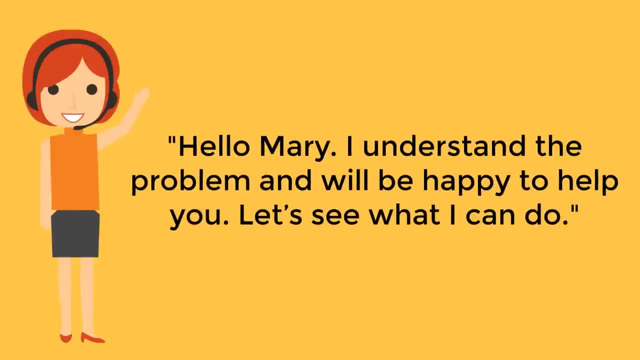 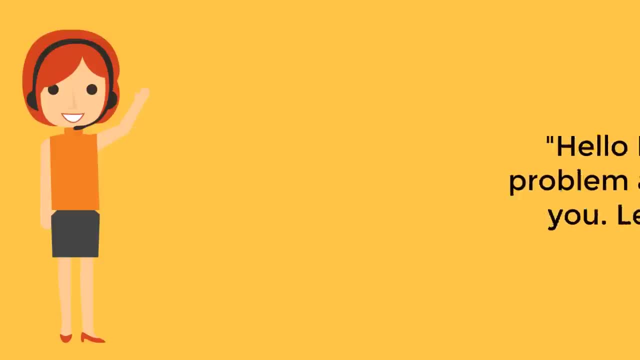 Hello Mary, I understand the problem and will be happy to help you. Let's see what I can do. If the customer did not provide his name, you can ask for it. It will show your concern and attention. Hello, may I have your name please? 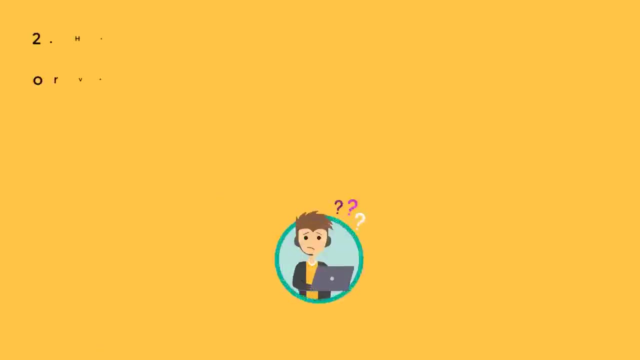 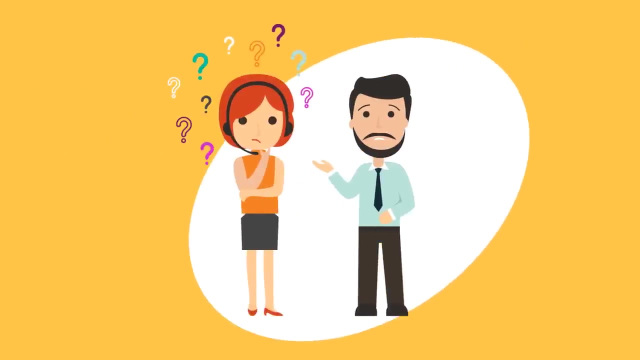 Once you have the name, make sure to spell it correctly: How to ask for more information or verify your understanding of the question or problem. To avoid any confusion and a long chat, make sure you understand the customer's issue before giving your instructions or offering solutions. 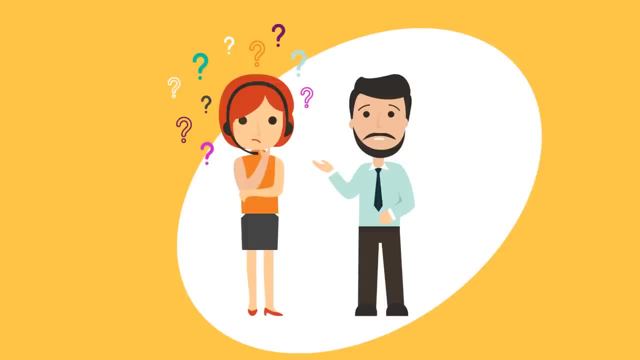 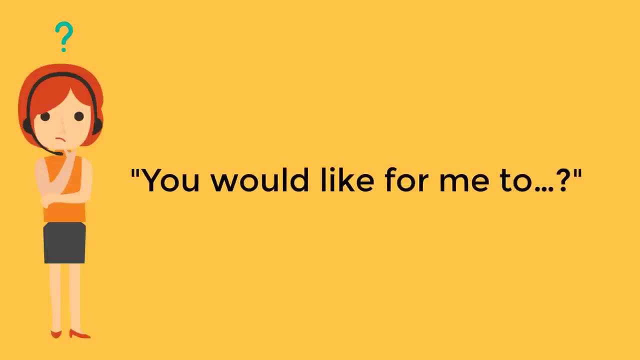 There are many ways you can ask for clarification. politely, Let me check if I have this right. Let me see if I have this correct. You want me to… Or you would like for me to…, If I understand you correctly, Tell me more about…. 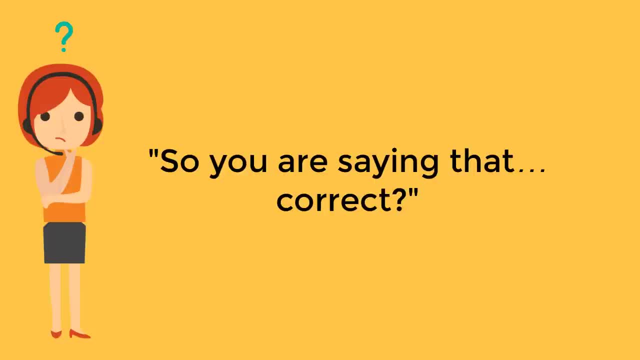 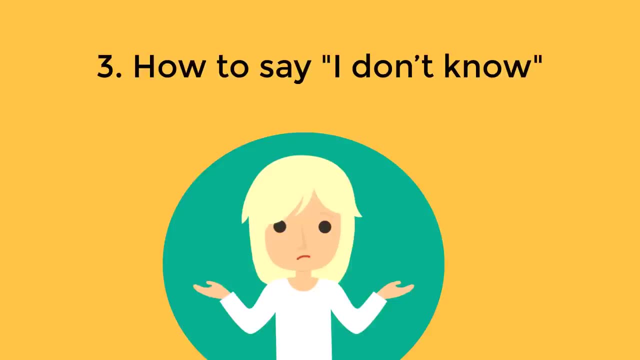 So you are saying that… Correct, This is what I understand. you are telling me How to say I don't know. If you don't know the answer to the customer's questions, be frank about it. However, avoid using the too straightforward I don't know. 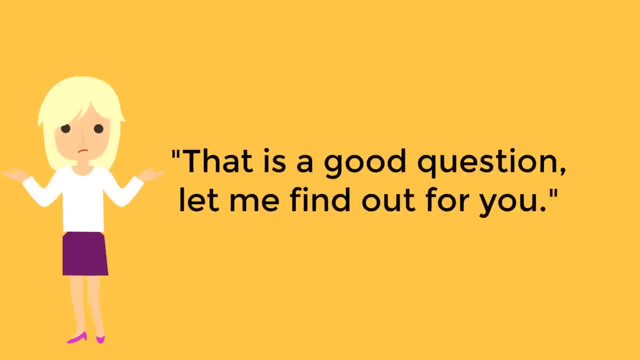 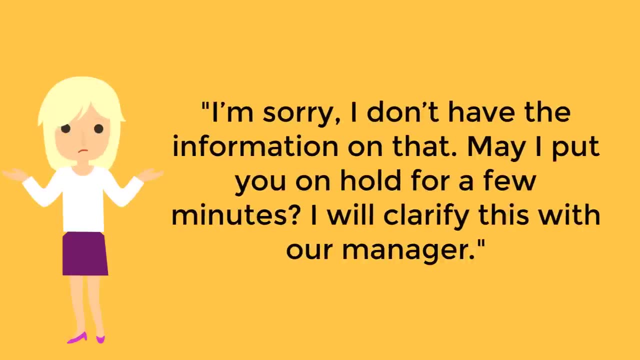 Here's how you can play it out. nice, That is a good question. Let me find out for you. I'm not sure, but let me find out for you. I'm sorry, I don't have the information on that. May I put you on hold for a few minutes? I will clarify this with our manager. 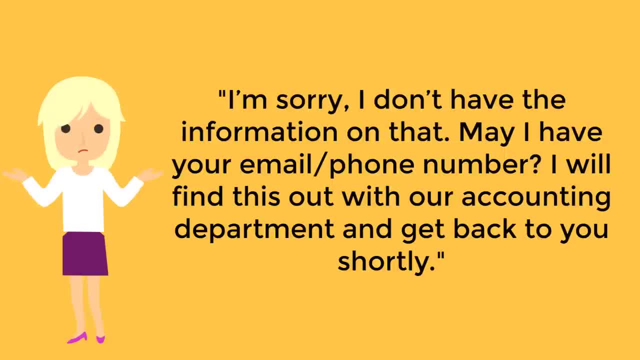 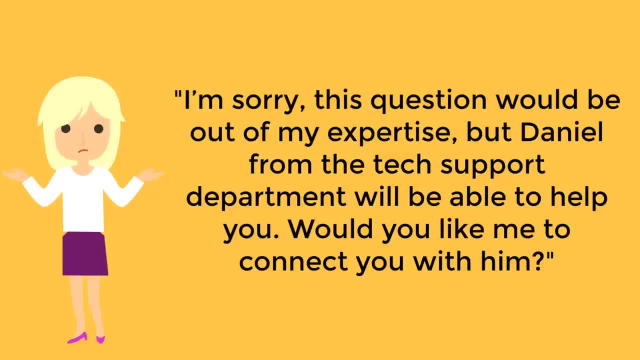 I'm sorry I don't have the information on that. May I have your email or phone number? I will find this out with our accounting department and get back to you shortly. I'm sorry this question would be out of my expertise, but Daniel from the tech support department will be able to help you. Would you like me to connect you with him? 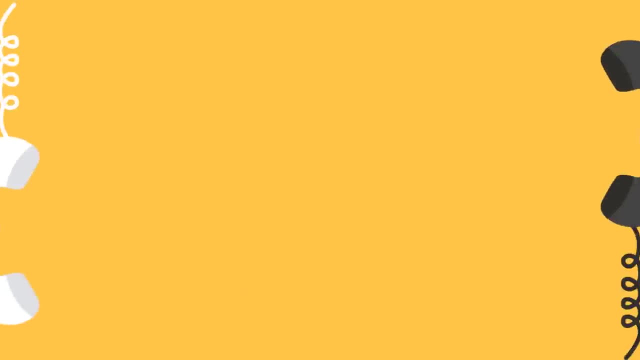 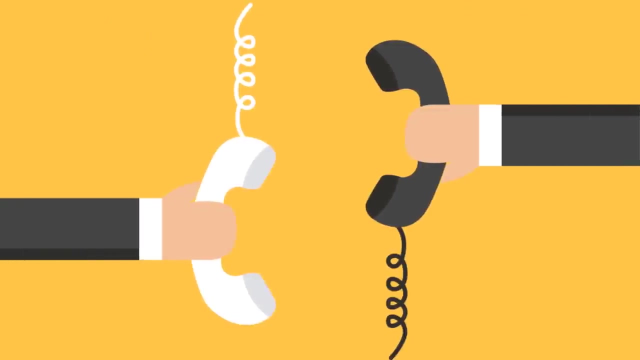 How to transfer. It is no secret that most customers do not enjoy being transferred. So if you have to transfer, do it only when it's absolutely necessary. Otherwise, try to find out the information for yourself Before transferring. inform the customer why and to whom their call is being transferred. 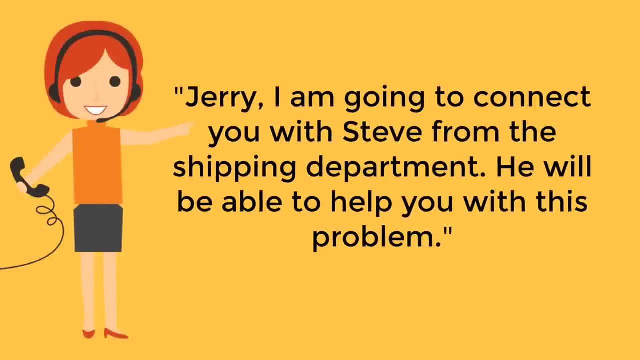 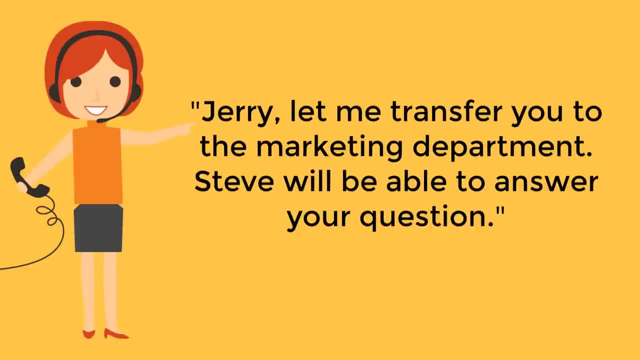 Jerry, I am going to connect you with Steve from the shipping department. He will be able to help you with this problem. Jerry, let me transfer you to the marketing department. Steve will be able to answer your questions. Okay, Steve will be able to answer your question. 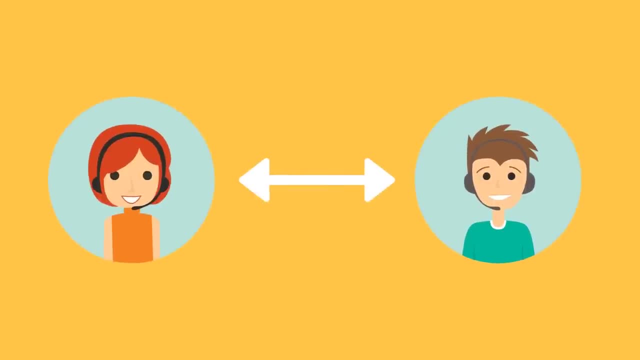 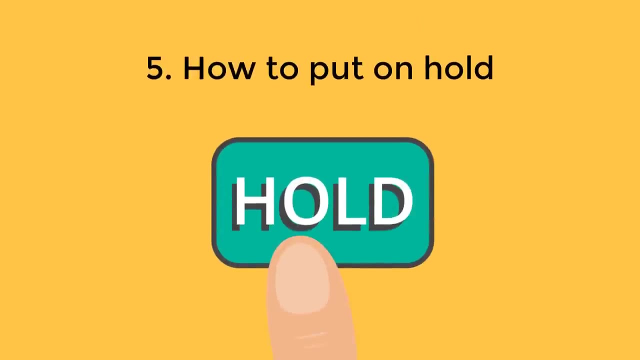 It is also important to notify the person to whom you are transferring the chat. Give them the customer's name and explain the nature of their question or problem. How to put on hold. If you need some time to investigate the problem, ask the customer's permission to put them on hold. 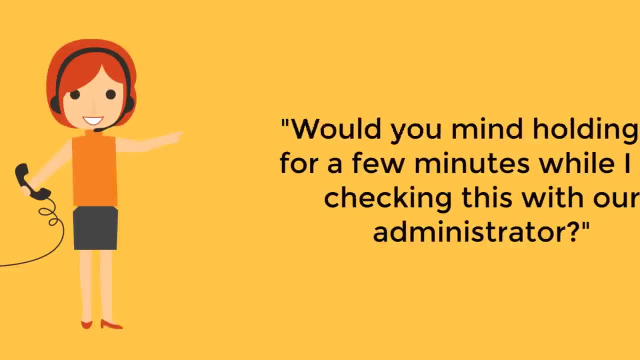 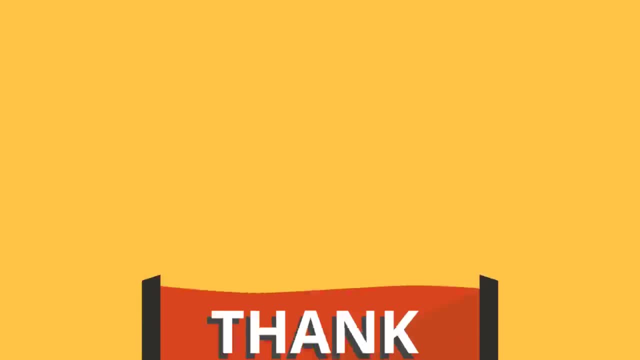 Would you mind holding on for a few minutes while I'm checking this with our administrator? May I put your call on hold while I'm checking your order, Can I put you on hold for a moment On receiving their consent. make sure to thank the customer before leaving the chat. 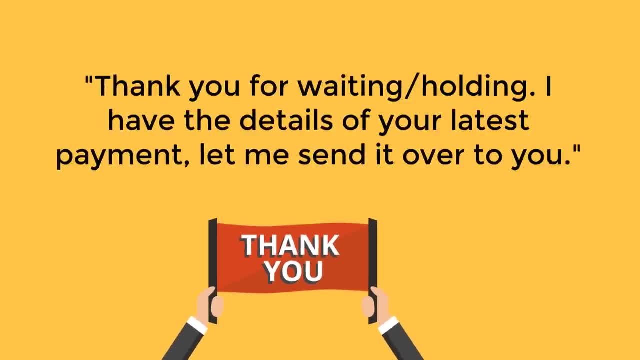 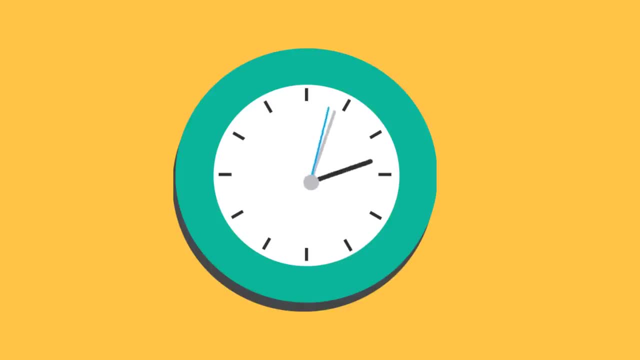 When you are back. thank them again for waiting. Thank you for waiting or thank you for holding. I have the details of your latest payment. Let me send it over to you. If you feel resolution of their problem is going to take a longer time, ask the customer whether they would like you to call or email them back rather than waiting on hold. 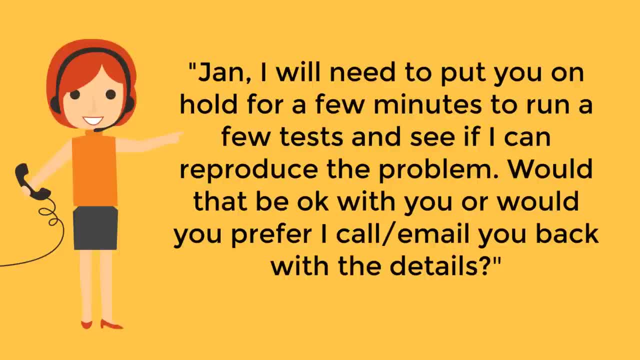 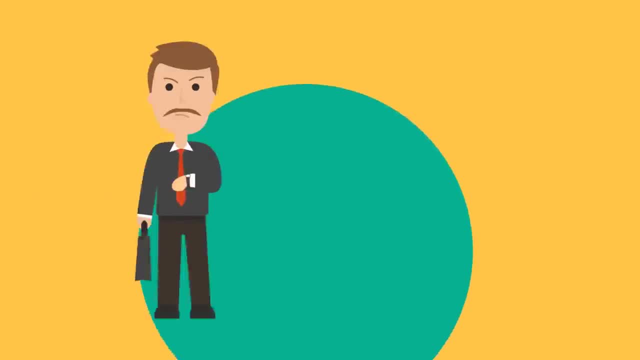 Jen, I will need to put you on hold for a few minutes to run a few tests and see if I can reproduce the problem. Would that be okay with you, or would you prefer I call or email you back with the details? If you have been away for too long and the customer has been inquiring about your absence, make sure to apologize to them. 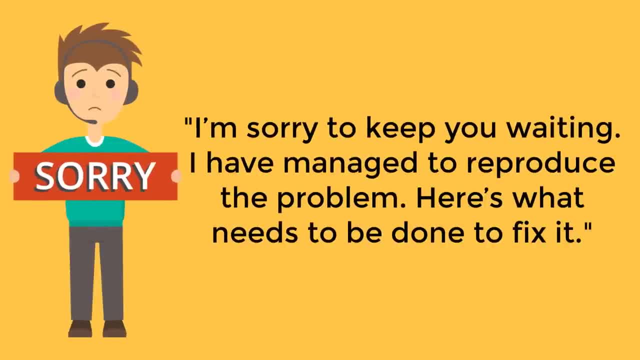 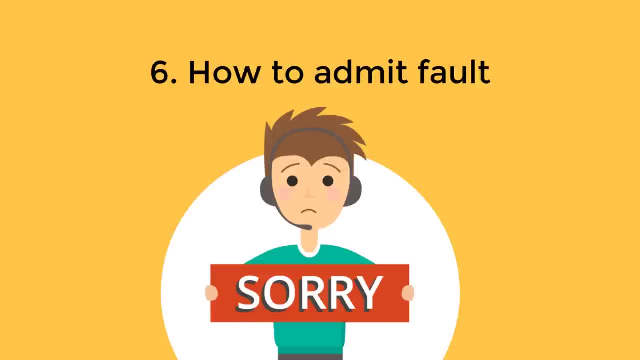 I'm sorry to keep you waiting. I have managed to reproduce the problem. Here's what needs to be done to fix it. How to admit fault. Be direct and clear about the fact that you made a mistake. If it is your personal fault, do not admit it. 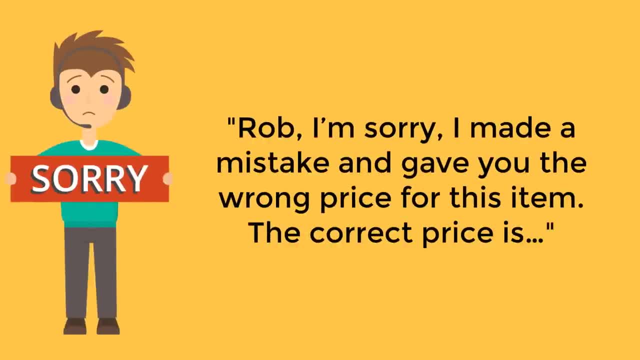 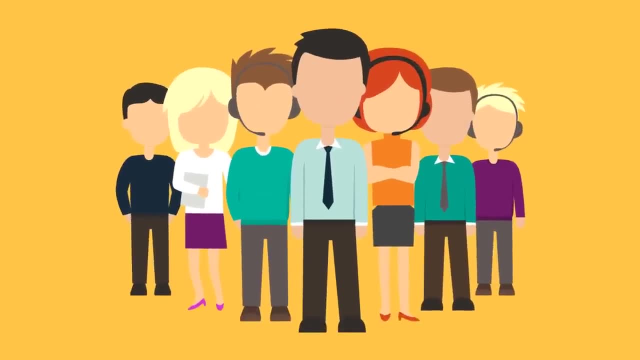 If it is your personal mistake, say that. Rob, I'm sorry, I made a mistake and gave you the wrong price for this item. The correct price is: If it is someone else's mistake, say that it was our mistake, attributing it to the company rather than to the individual person who is not present in the chat room with you. 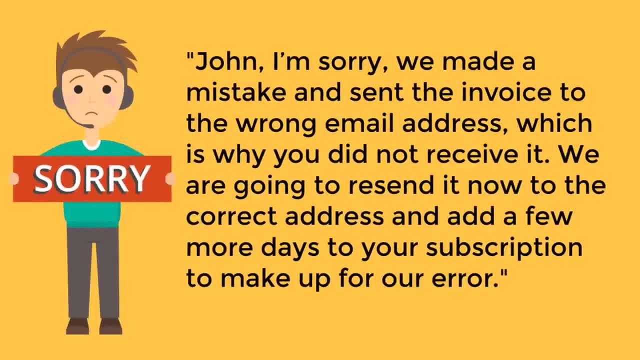 John, I'm sorry. we made a mistake and sent the invoice to the wrong email address, which is why you did not receive it. We are going to resend it now to the correct address and add a few more days to your subscription. How to make up for our error. 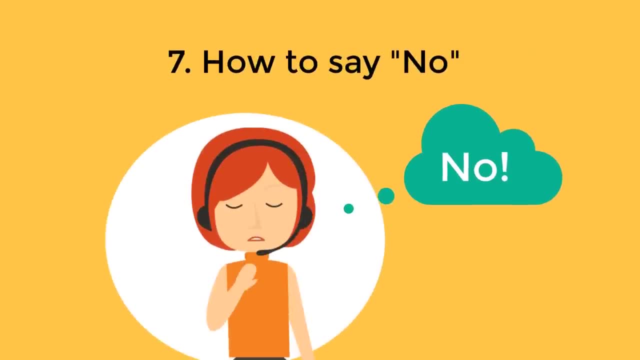 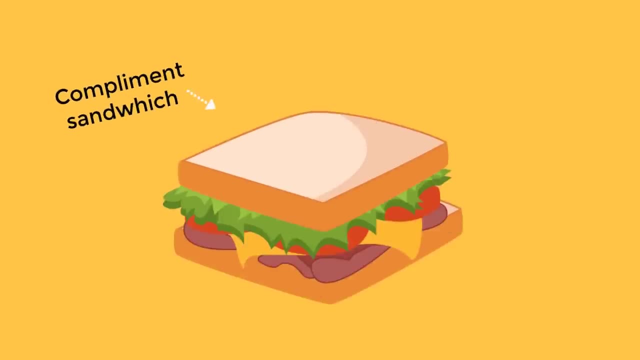 How to say no. Saying a blank no to the customer may appear quite rude. The best approach is to use the compliment sandwich, a great tactic which John Rydell beautifully describes in his article Simple Tips on Having the Hard Conversation. This tactic is basically about adding two positive statements on either side of a bad one. 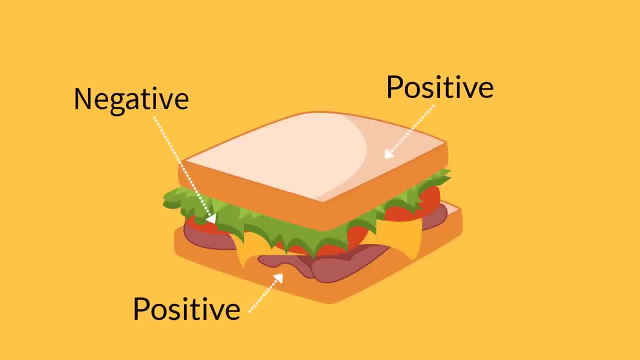 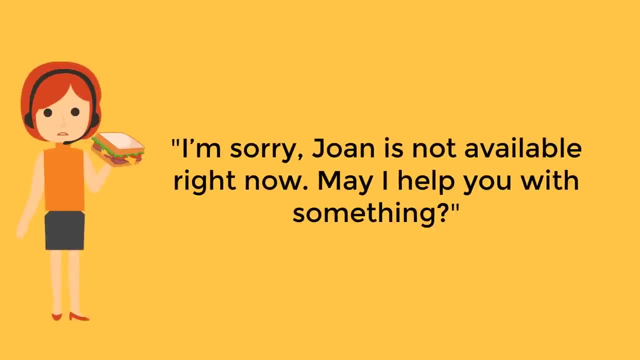 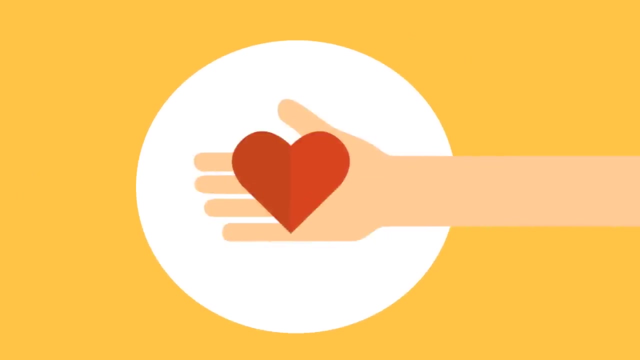 For example, if the customer is asking to be connected with a team member who is not available for a chat, you would usually say: I'm sorry, Joan is not available right now. may I help you with something? First, you express empathy that the customer's desire cannot be fulfilled at the moment. 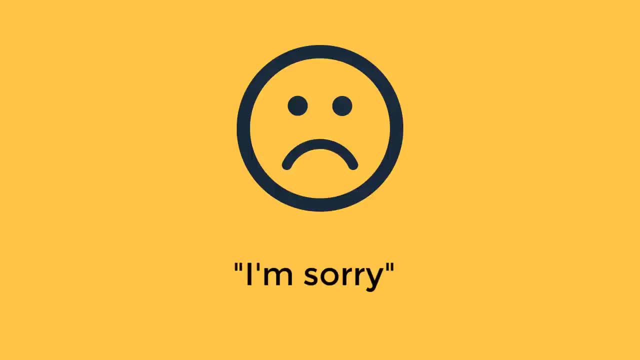 I'm sorry. Then you make the actual negative statement. Joan is not available. After that, you complete your response with something positive, an offer of help. May I help you with something? You could extend this to deal with more complicated situations. 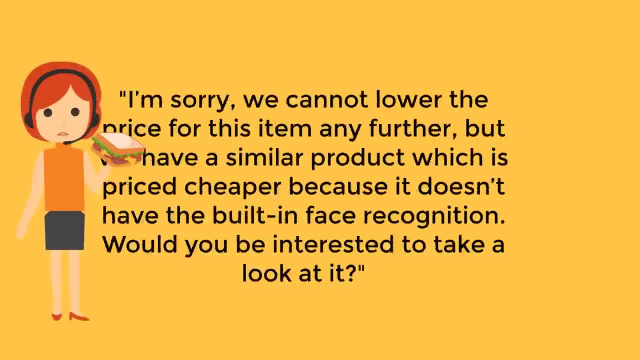 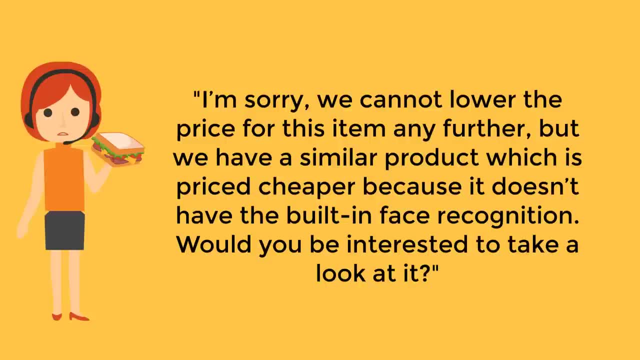 Here are a few more examples. I'm sorry we cannot lower the price for this item any further, But we have a similar product which is priced cheaper because it doesn't have the built-in face recognition. Would you be interested to take a look at it? 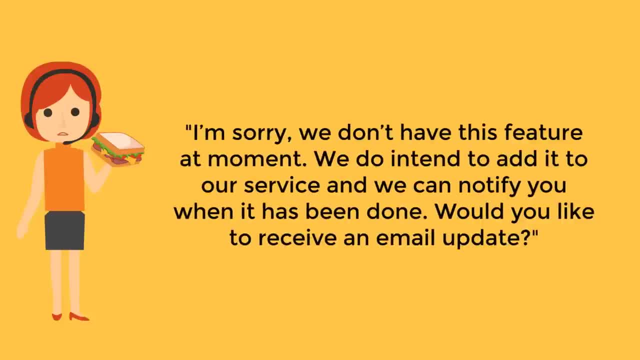 I'm sorry we don't have this feature at the moment. We do intend to add it to our service and we can notify you when it has been done. Would you like to receive an email update How to follow up If you promise the customer to call or email them back? 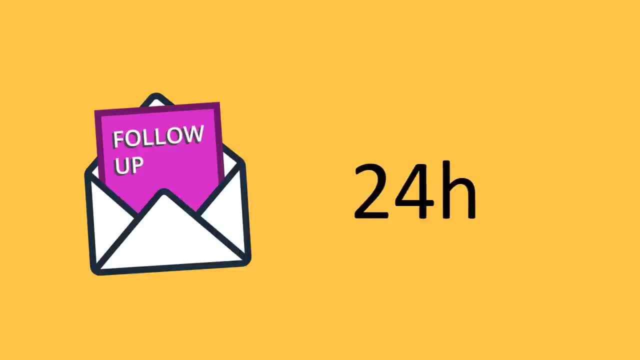 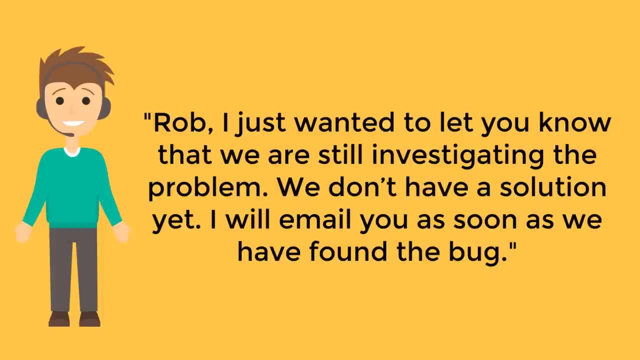 it is desirable that you do that within a 24-hour time frame, even if you don't have an answer to their question yet. Rob, I just wanted to let you know that we are still investigating the problem. We don't have a solution yet. 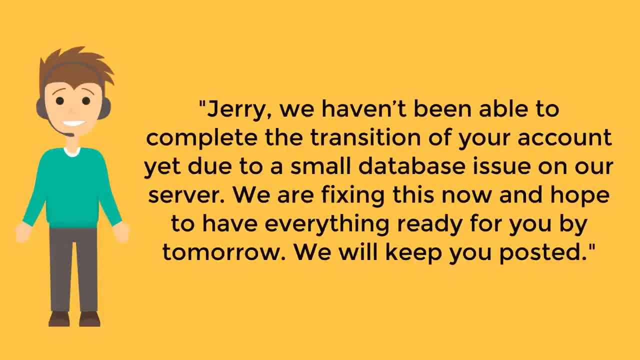 I will email you as soon as we have found the bug. Jerry, we haven't been able to complete the transition of your account yet due to a small database issue on our server. We are fixing this now and hope to have everything ready for you by tomorrow. 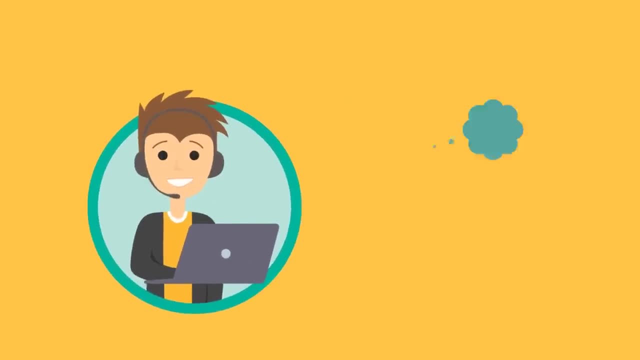 We will keep you posted. If you missed a chat request and have the customer's contact information, your client will no doubt appreciate it if you follow up with them right away. Hello Tom, I'm sorry we have missed your chat. Is there anything we can help you with? 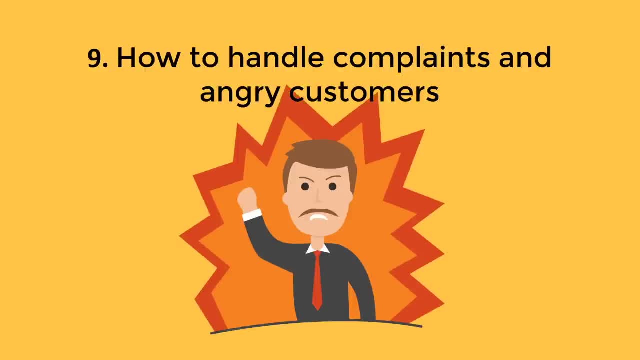 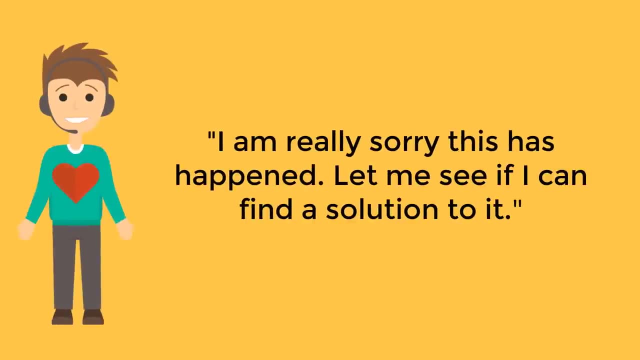 How to handle complaints and angry customers. Start by showing sincere sympathy and understanding. Acknowledge the customer's feelings. I am really sorry this has happened. Let me see if I can find a solution to it. I'm really sorry about that. Tell me what happened. 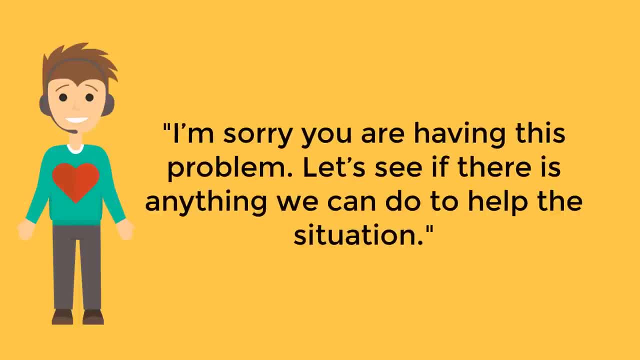 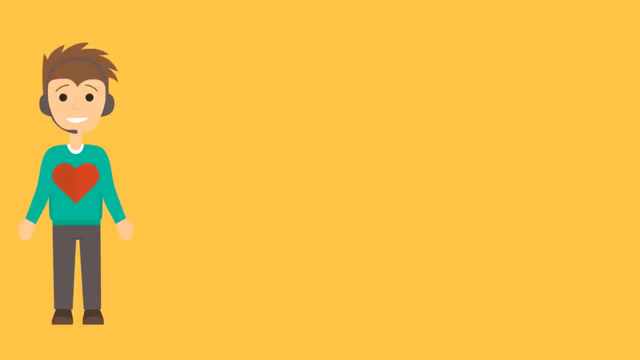 I'm sorry you are having this problem. Let's see if there is anything we can do to help the situation. Express your willingness to help commit till you find a solution or compromise to deal with the issue. I'm sorry you are not happy with our product or with your purchase. 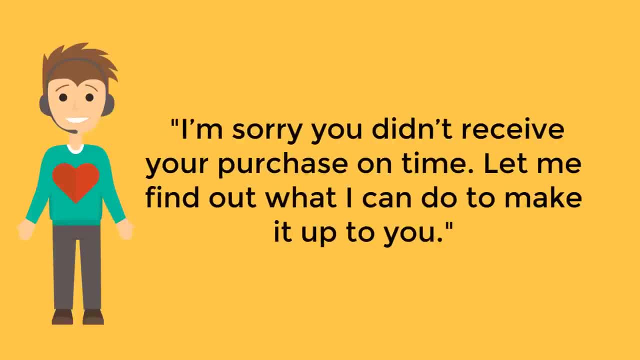 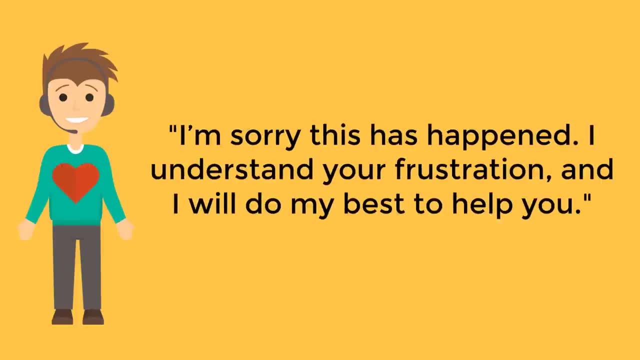 Let's see what we can do to make things right. I'm sorry you didn't receive your purchase on time. Let me find out what I can do to make it up to you. I'm sorry this has happened. I understand your frustration and I will do my best to help you. 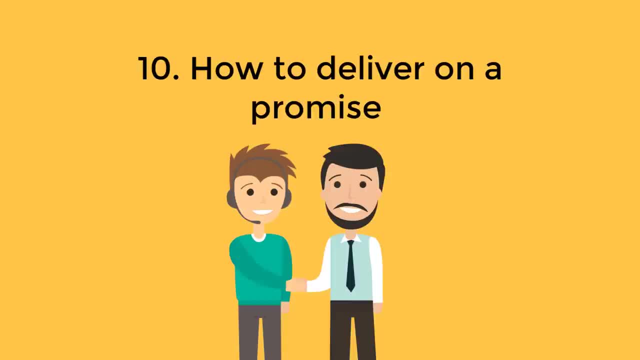 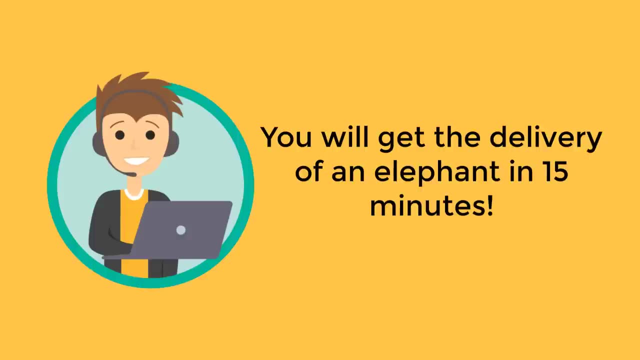 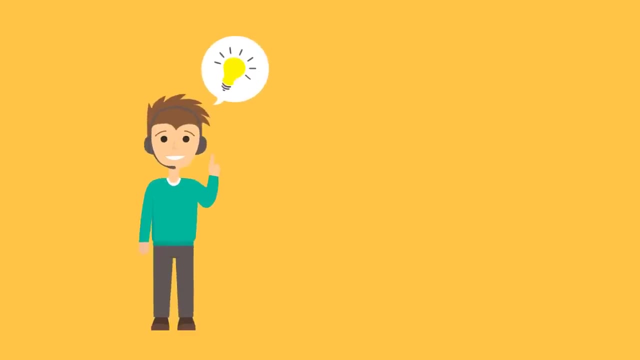 How to deliver on a promise. Sometimes it happens that a customer has been promised something which is impossible to accomplish, either through lack of knowledge or misinformation. Instead of direct denial- we could not have promised anything like that- Reassure the customer that you are going to verify that which he had been promised and offer him apologies if there was a mistake. 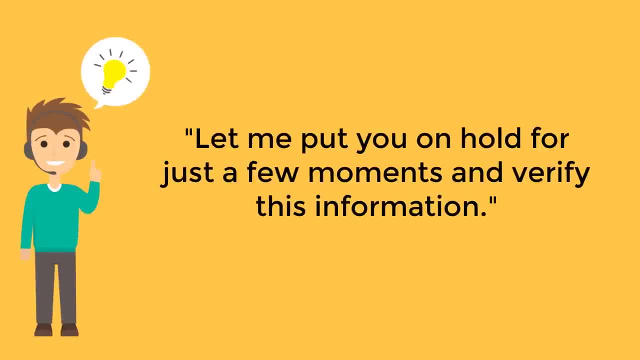 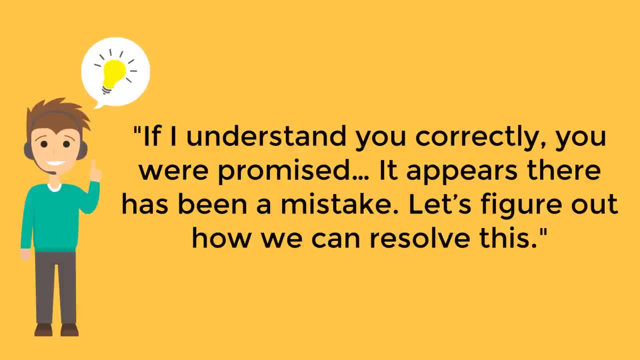 Let me put you on hold for just a few moments and verify this information. If I understand you correctly, you were promised… It appears there has been a mistake. Let's figure out how we can resolve this. How to handle several clients simultaneously. 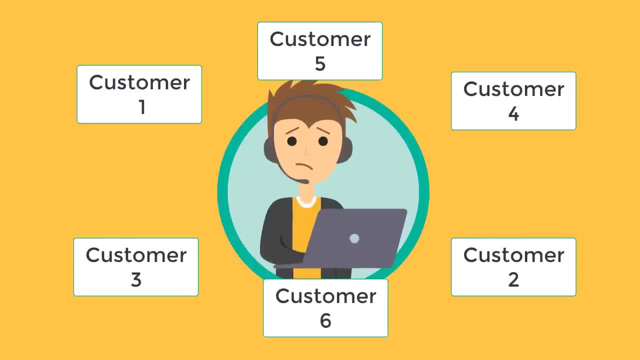 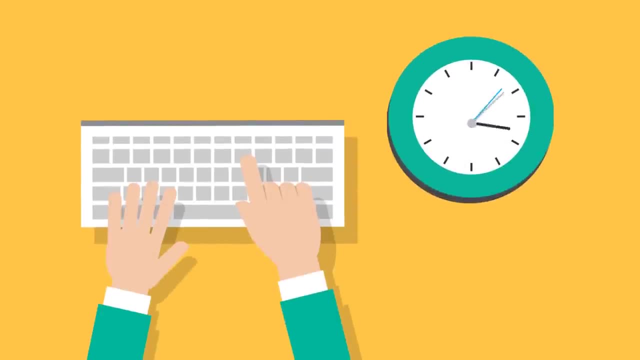 When you have to deal with several clients at the same time, do not give the impression that you are rushed. If it is necessary, take the extra time for yourself by telling the customer that you are going to check the information for him And asking him to hold for a few minutes. 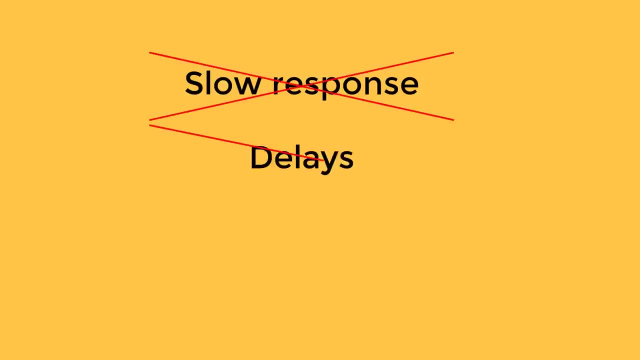 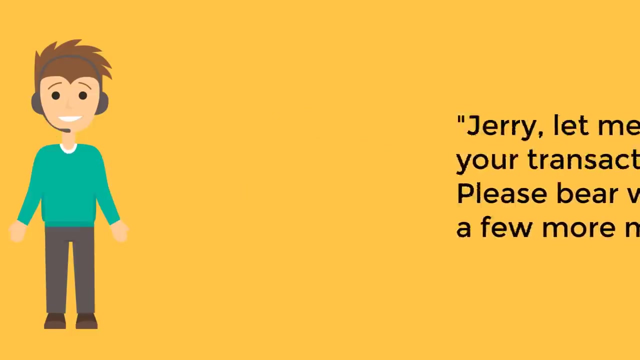 The customer is not concerned with slower responses or minor delays. They are concerned with lack of your attention. It is okay to make them wait if you first ask their permission for it. Jerry, let me review your transaction history. Please bear with me for a few more minutes. 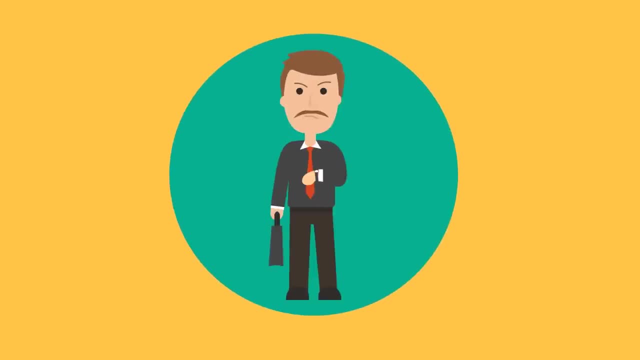 If your responses are delayed and the customer inquires about it, never tell them you are dealing with other clients. The customer should always have the impression that he is the only one you are dealing with at that moment. If there are delays, attribute them to your checking up the information for the client. 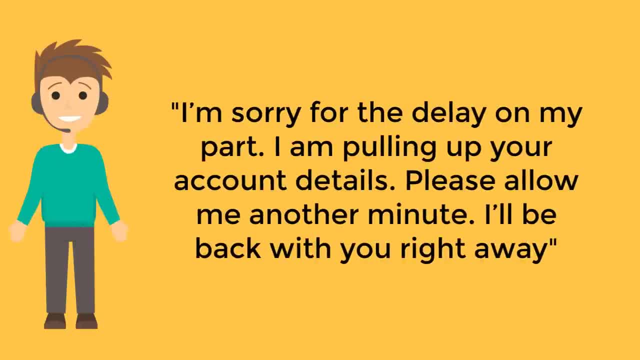 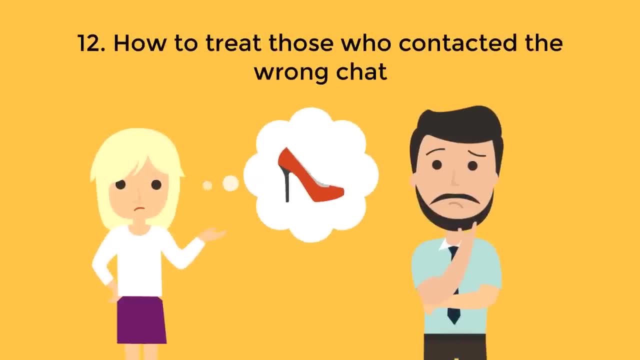 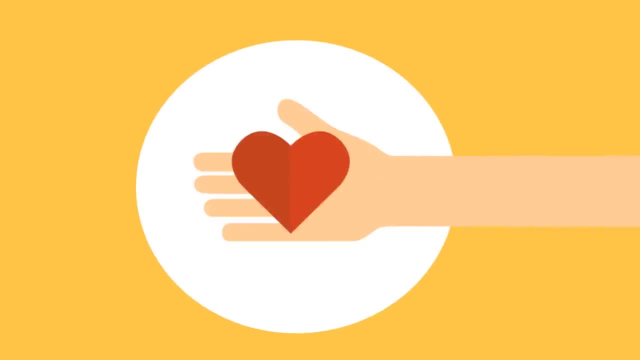 I am sorry for the delay on my part. I am pulling up your account details. Please allow me another minute. I will be back with you right away. How to treat those who contacted the wrong chat. It is important to treat all callers with respect, even if they are not your clients or participants. 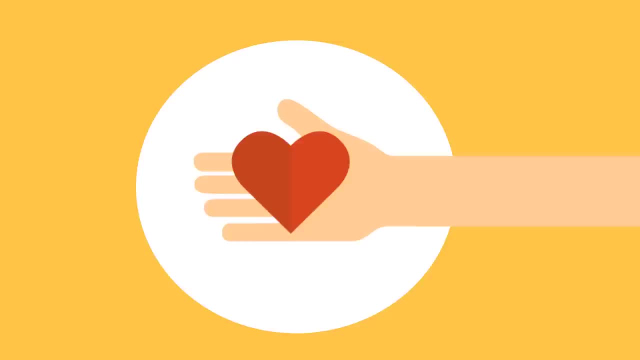 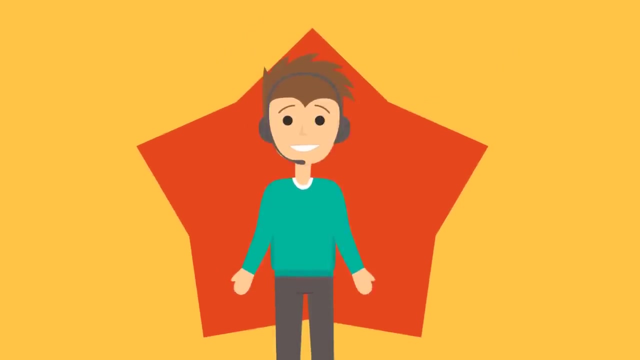 Most people who are contacting you by chat have some sort of online presence, And if you are rude with them or reluctant to give them a clear answer, they can leave false, negative comments about your company in online forums or on social media. To avoid such situations, make sure to come up with a friendly response to such callers. 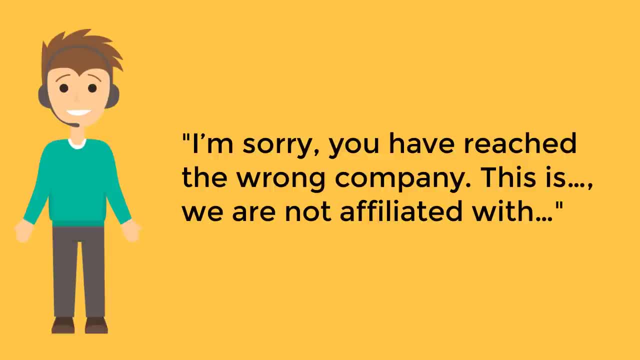 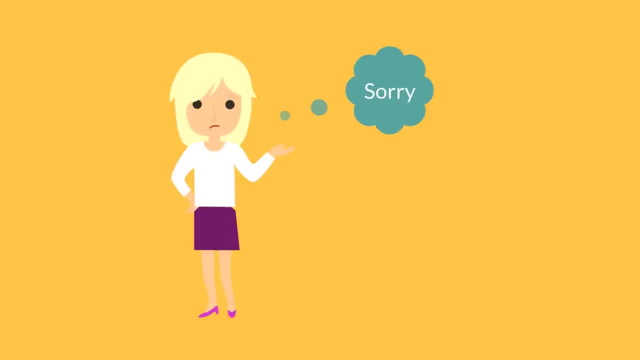 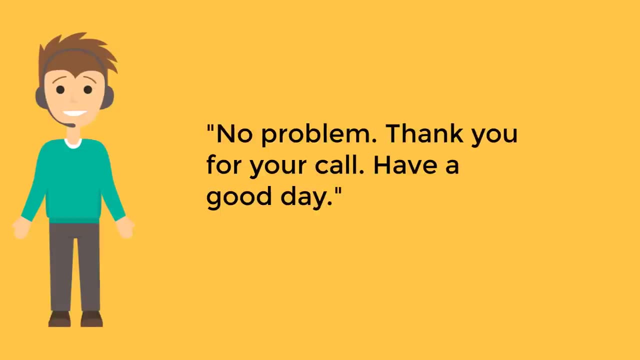 I am sorry you have reached the wrong company. This is…. We are not affiliated with…. If they apologize for having reached the wrong chat, reassure them everything is okay and end the chat, No problem. Thank you for your call. Have a good day.